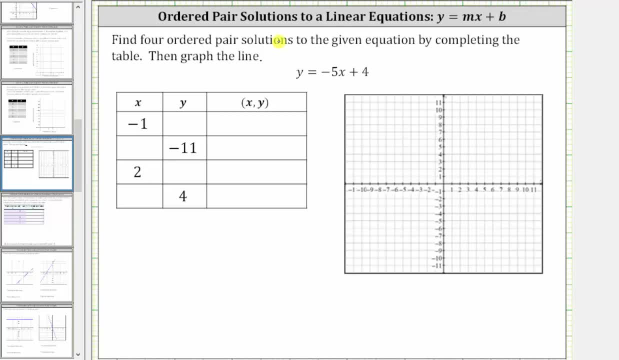 We're asked to find four ordered pair solutions to the given equation by completing the table, then graph the line. The equation is: y equals negative five x plus four. Looking at the first row, we are given x equals negative one To find the corresponding y value. 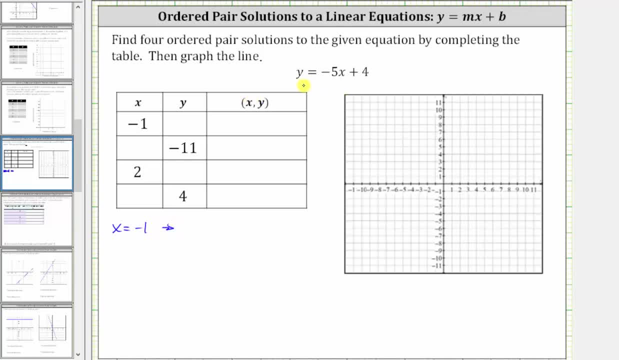 we substitute negative one for x and solve for y. Performing the substitution gives us y equals negative five times x, but x is negative one, giving us negative five times negative one. and then we have plus four, Simplifying on the right side. 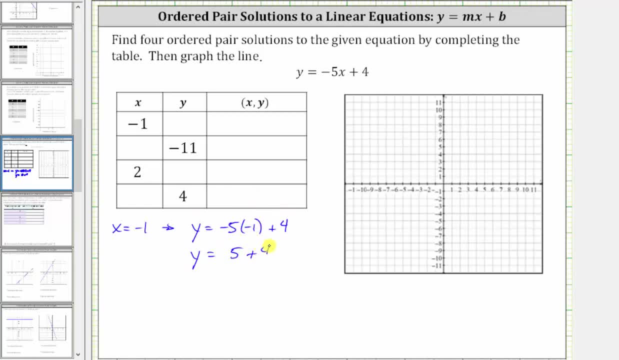 negative five times negative. one is positive five, and five plus four is equal to nine. When x is negative, one, y is nine. One ordered pair solution is negative, one comma nine. In the next row we are given: y equals negative 11,. 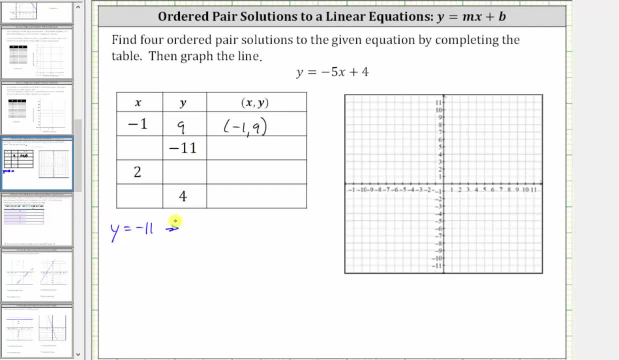 so now we substitute negative 11 for y and solve for x. Performing the substitution gives us the equation: negative 11 equals negative five x plus four. The first step is to add or subtract, to isolate the variable term. To undo the plus four, we subtract four on both sides. 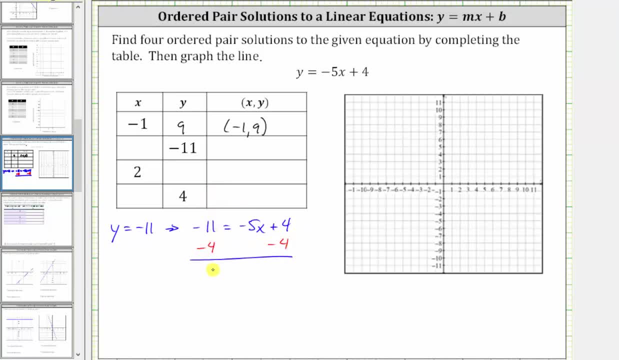 Simplifying negative: 11 minus four is negative 15.. On the right, four minus four is zero. The right side simplifies to negative five x. The next step is to multiply or divide to solve for x. Negative five x means negative five times x. 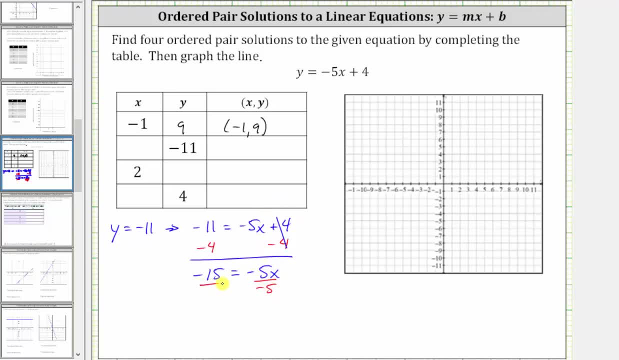 To undo the multiplication solve for x. To undo the multiplication solve for x. To undo the multiplication solve for x. We divide both sides by negative five. Simplifying negative 15 divided by negative five is three On the right. negative five divided by itself. 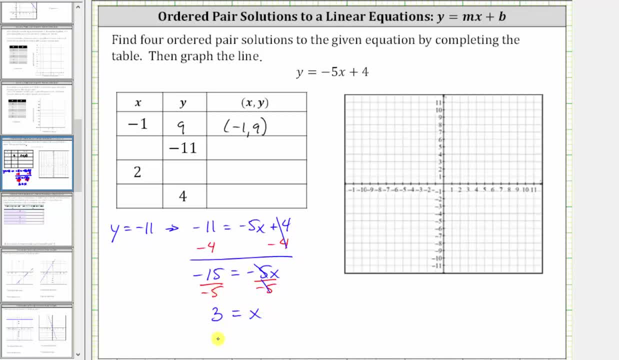 simplifies to one. One times x is x, Three equals x is the equivalent to x equals three. When y is negative 11, x is equal to three, The ordered pair solution is three comma negative 11.. In the next row, x equals two. 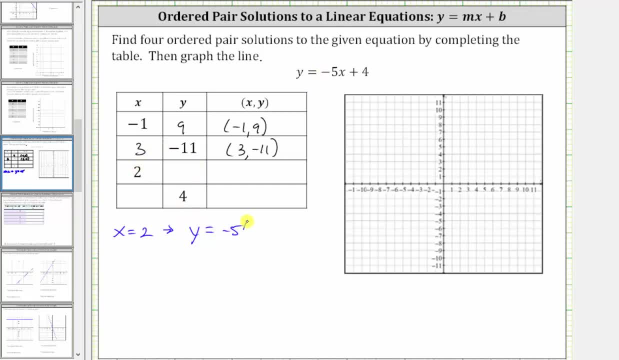 When x equals two, y, y is equal to negative five times two plus four. Simplifying negative five times two is negative 10.. And negative 10 plus four is equal to negative six. When x is two, y is negative six. 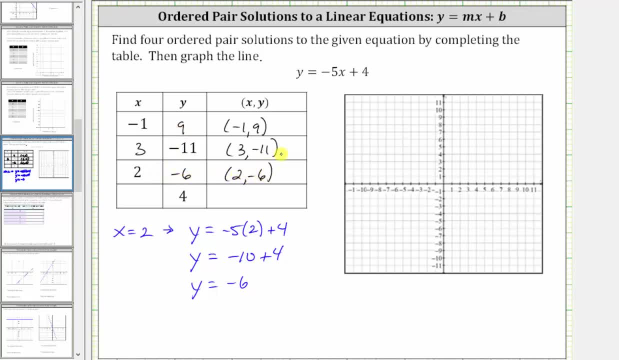 The ordered pair solution is two comma negative six And for the last row we are given y equals four. Substituting y for four gives us four equals negative five x plus four. First step: isolate negative five x by subtracting four on both sides. 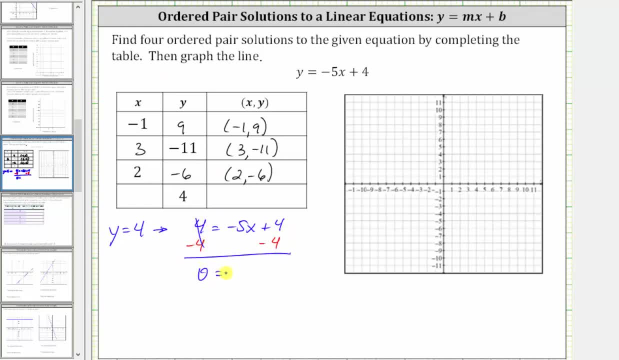 Simplifying: four minus four is zero. We have zero equals on the right: four minus four is zero. Again, the right side simplifies to negative five x. The last step to solve for x is to divide both sides by negative five. 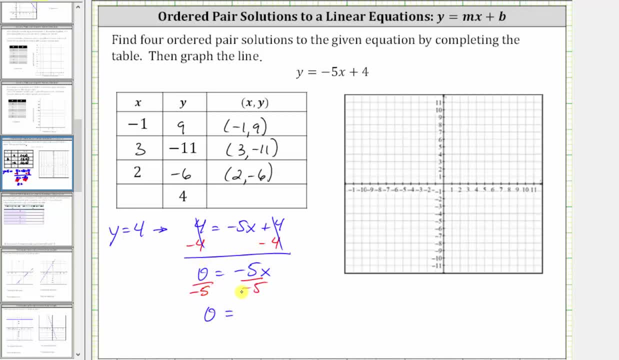 Simplifying: zero divided by negative five is zero. On the right, negative five divided by itself simplifies to one. One times x is x. Zero equals x is equivalent to x equals zero, which means when y is four, x is zero. 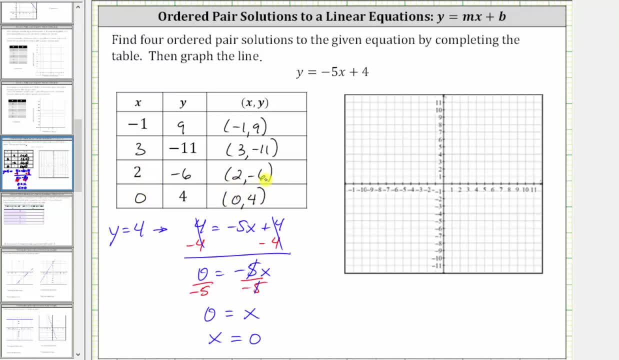 the ordered pair solution is zero comma four. And now to graph the line. we will graph these four points on the coordinate plane And if we found these ordered pairs correctly, a line will pass through all four points To plot the point negative one comma nine from the origin. 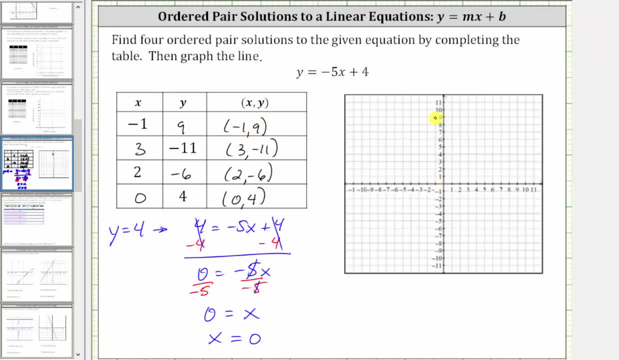 we move left one unit and then up nine units For three comma negative 11 from the origin. we move right three and then down 11 units. The next ordered pair solution is two comma negative six From the origin. we move right two units.